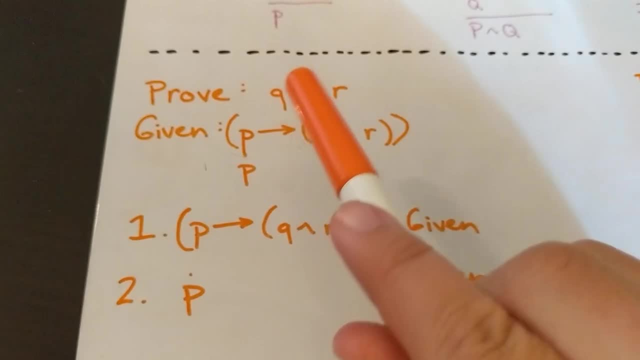 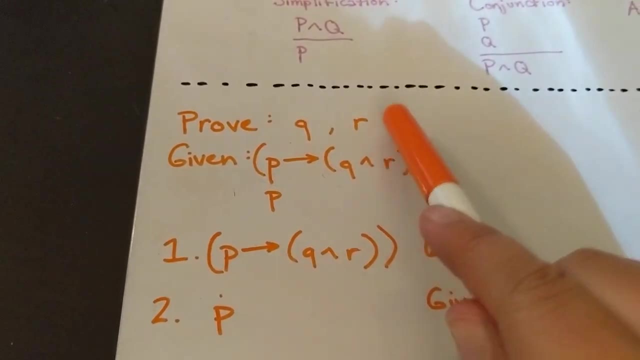 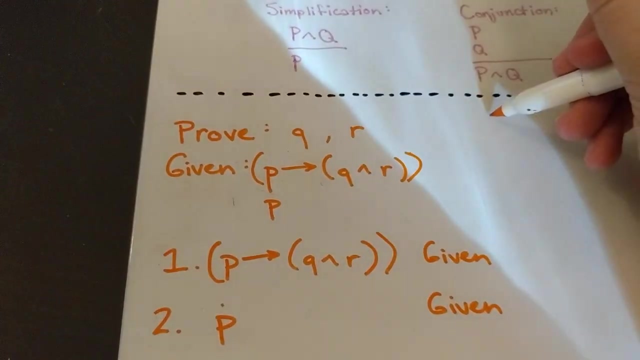 notice, though, is that when we're proving things using inference, usually it will say: prove q and r, and what that means is that q is true and r is true, And this just means that, if this comes from some ways that people view, models are, either you're in, 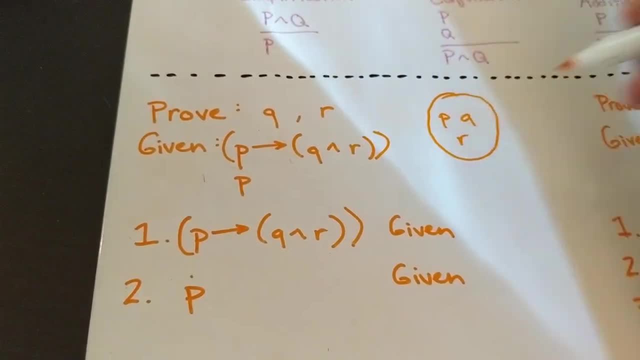 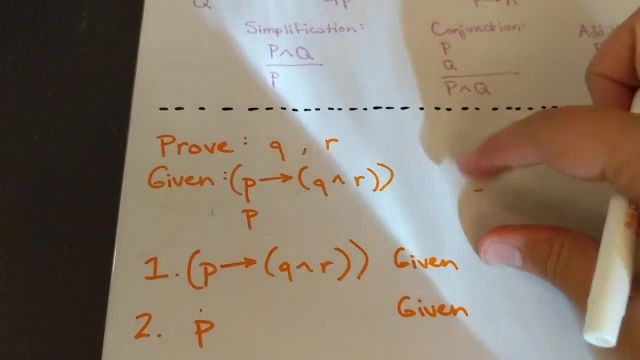 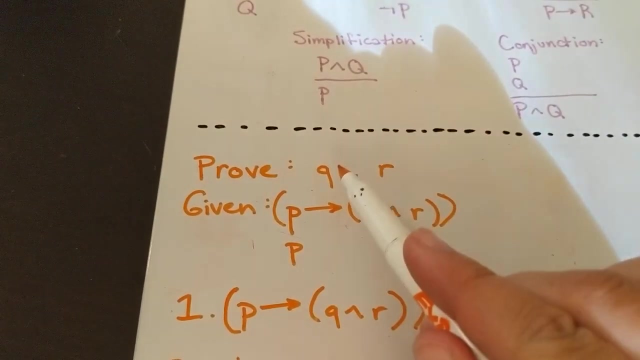 the model, in which case you're true, or you're outside of the model, in which case you're false. right, And so this comes from this way of viewing a model. but usually if you just see something listed like this, assume that means truth, right? So in our prove that in our model, q is true, and 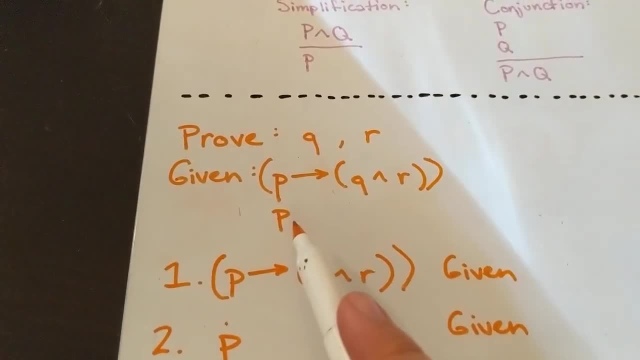 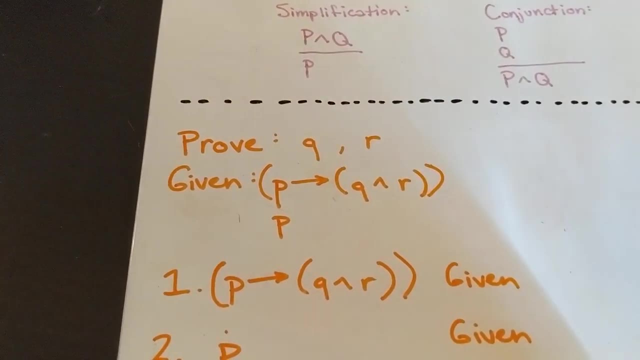 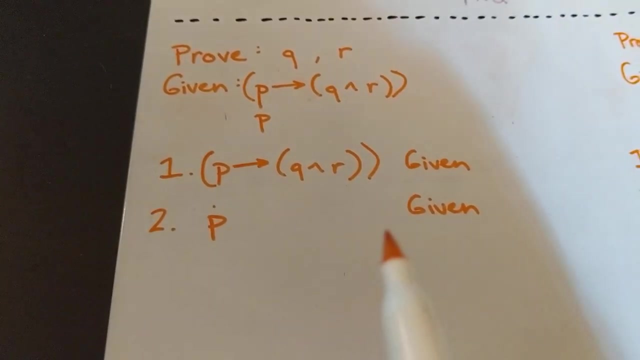 r is true, Given that in our model, p is true and in our model the statement p, if p, then q and r is also true, right? So that's what this statement means here. Okay, so our first two steps are to put down what we are given. So these are our two pieces of given information, and now we're going to start doing. 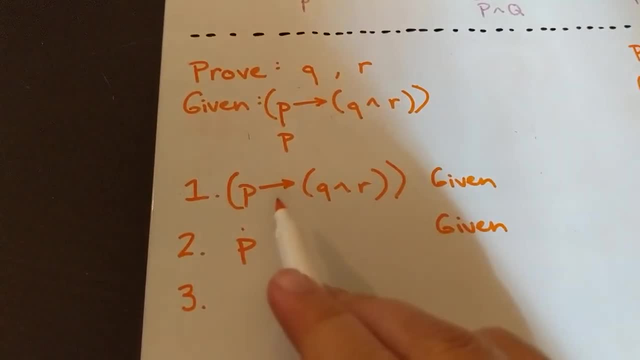 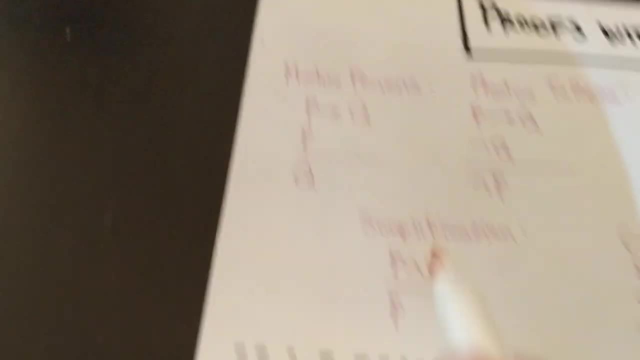 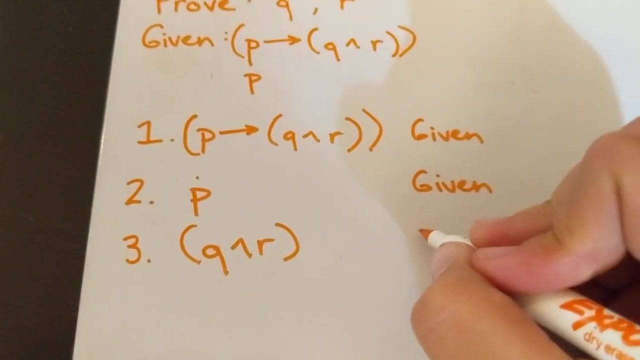 more things with that. So our first step, since this is a simple implication, is to look up to modus ponens. The left side is true, so we know that the right side is true, So we can conclude: q and r is true by modus ponens. 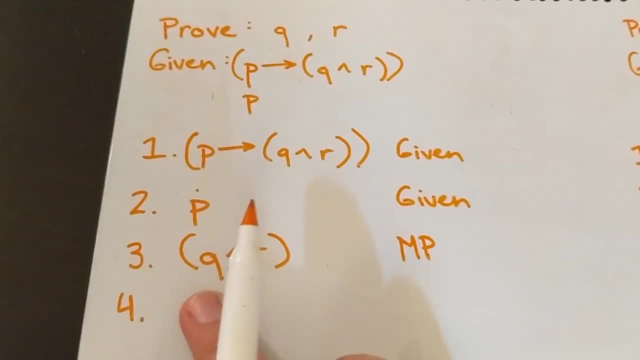 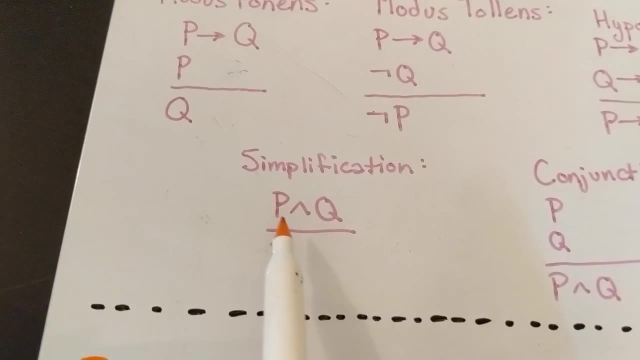 Our next step is going to be to conclude. we want to be able to conclude that q is true and r is true separately, And, luckily enough, we have this lovely little simplification rule that says that if the, and is true, then each one of those is true. 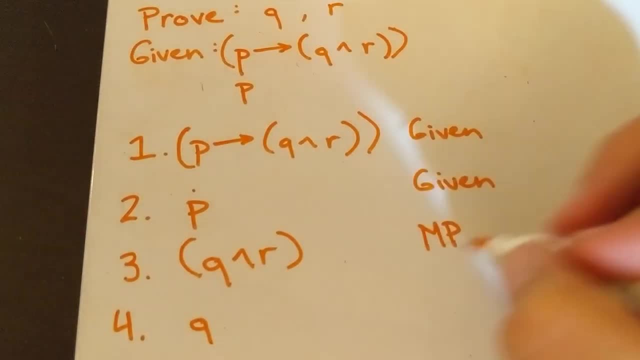 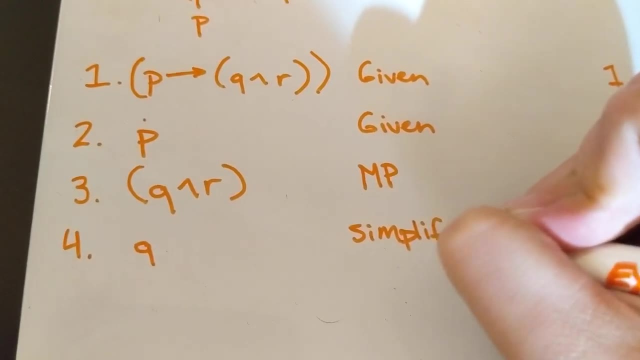 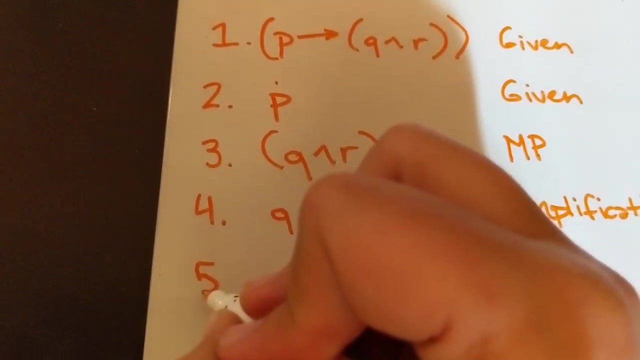 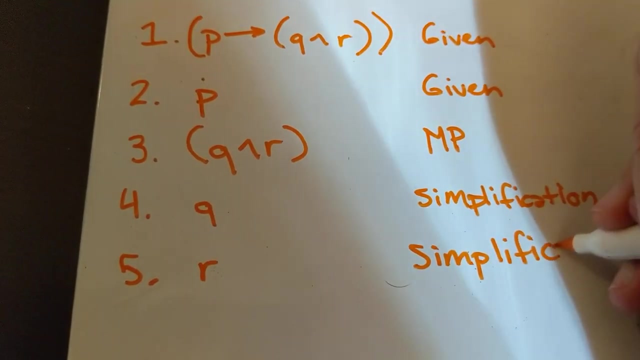 So we have to do this twice. So the first one, we conclude q based on simplification, And the second one, we're going to conclude that r is true based on simplification. So sometimes these proofs can look a little bit confusing because it's a little bit confusing. 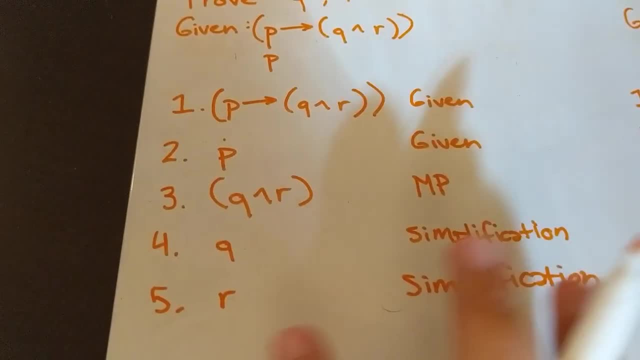 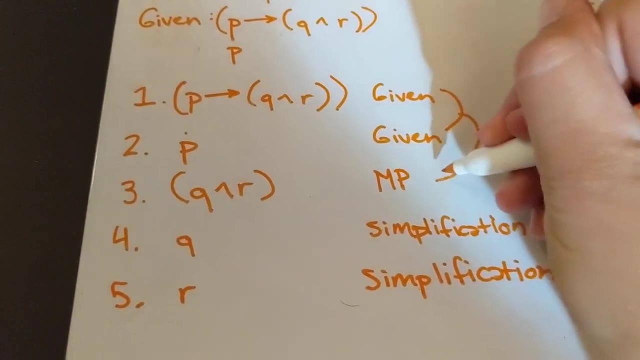 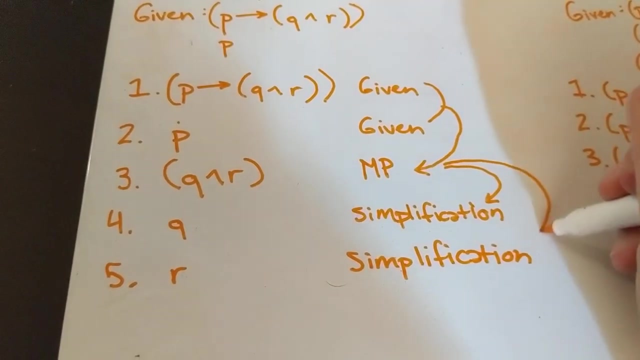 It's a little unclear what lines are going into each inference. So, for example, we are taking these two lines and putting them together for this one, And then for this one we just take this line and use it for simplification. And for this one we're taking this line and using it for simplification. 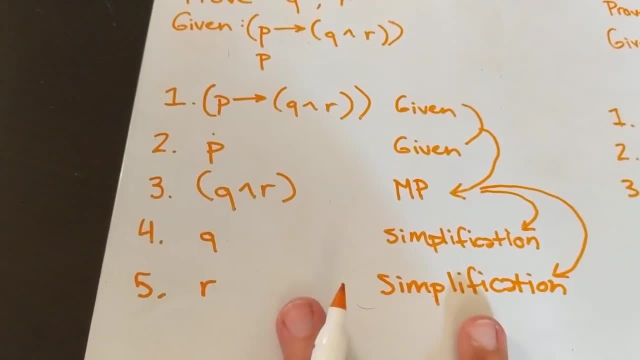 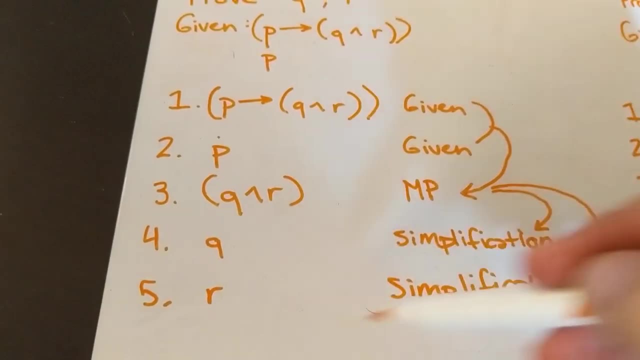 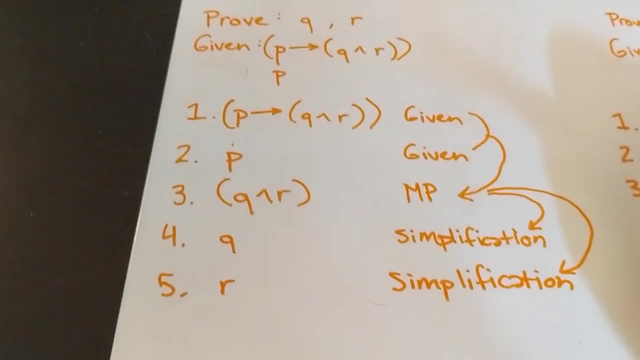 So it can get a little bit confusing to read and you may run into that problem when you're reading proofs given in the book. But just know that you can sort of hop along between different things, You can have different lines in a way that you can't with our simplifications using logic laws that we were doing before. 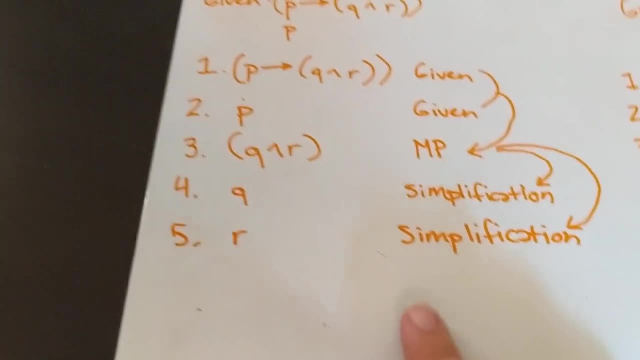 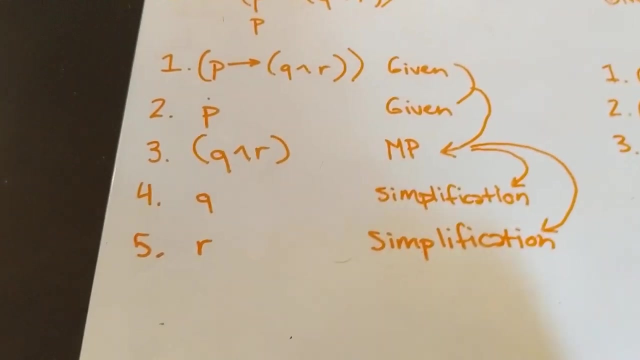 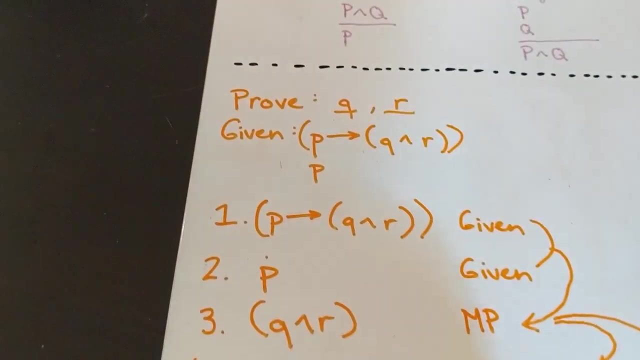 But you still have to have something above that you're using to conclude something below. It's not always just the line right above it, And so this can be hard to keep yourself organized as you're doing these proofs. But here we have concluded that q is true and r is true, which was our goal. 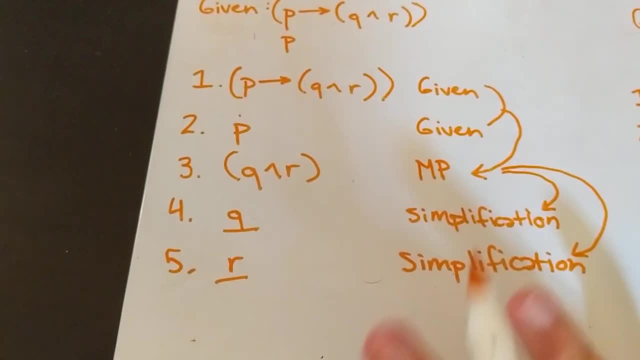 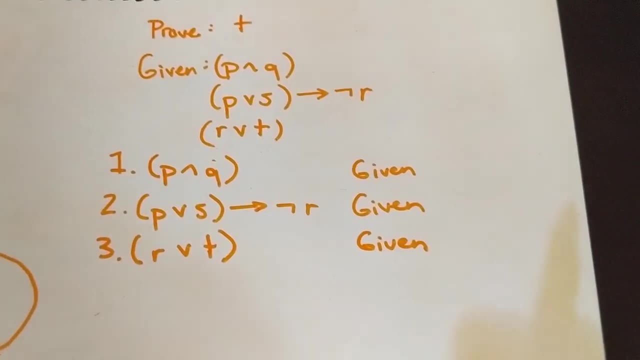 And so we are done with that proof. It's not a very long proof. It gives you an idea of how this works. We're going to do one more on this video and then we'll start mixing our logic laws with the rules of inference in the next video. 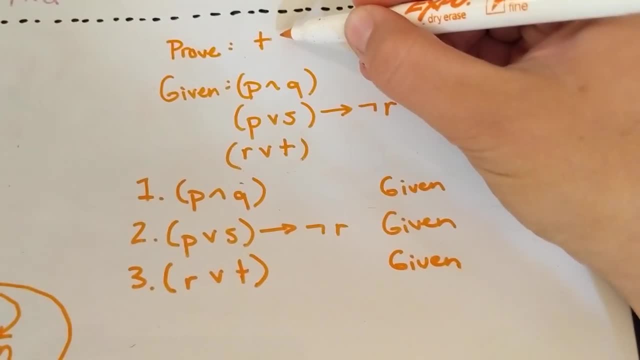 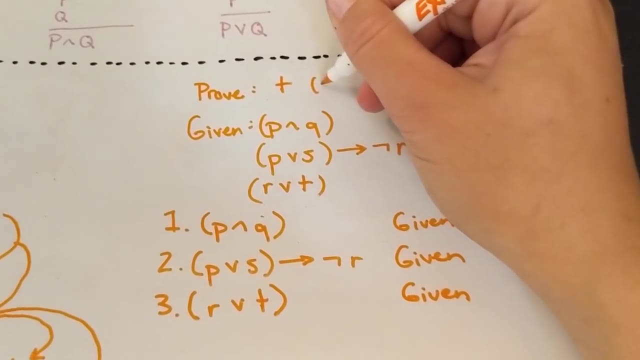 So in this one we are being asked to conclude that t is true in our model. So prove t is true. So when somebody says, prove t is true, is what you want to think in your head. I'm going to erase that, just because it's confusing. 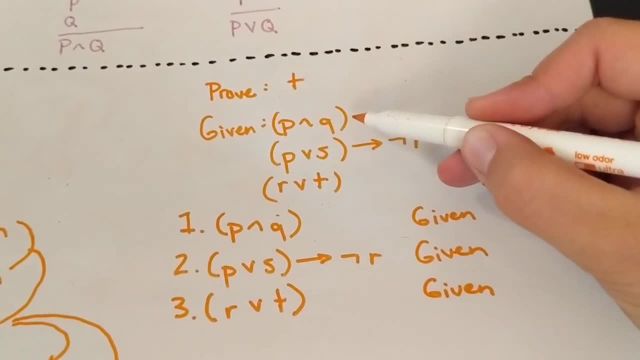 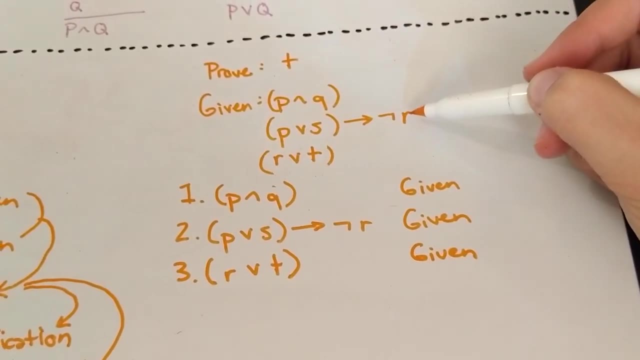 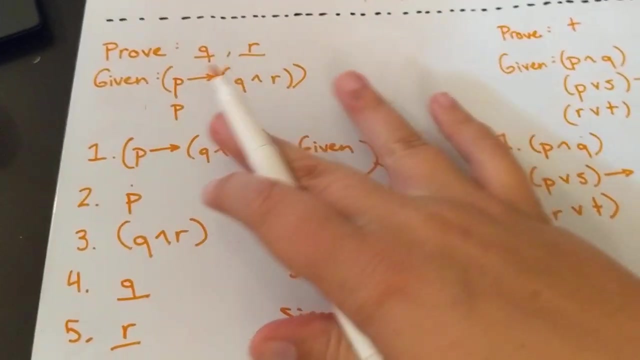 But that's what you want to think in your head. Given that p and q is true, p or s implies not r is true and r or t is true. So this is a little bit less transparently obvious than this, But it's actually fairly easy to prove, given these givens. 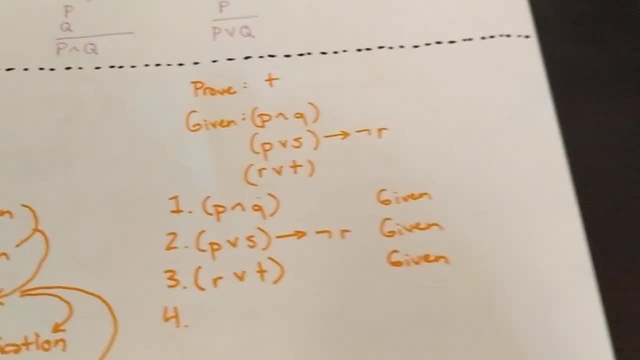 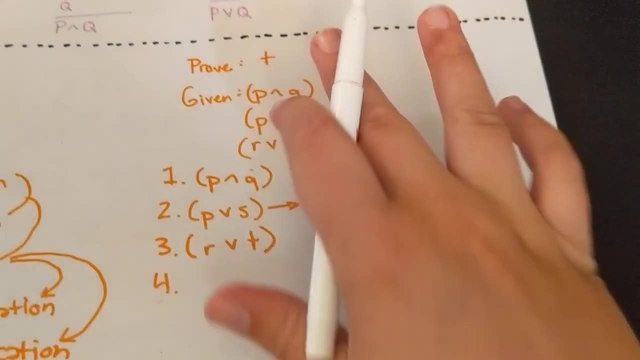 All right. So our first step, which is step number four, So our first step is to write out our givens, And then we want to start moving toward this, We want to start moving toward statements about t, So we're going to start with this one. 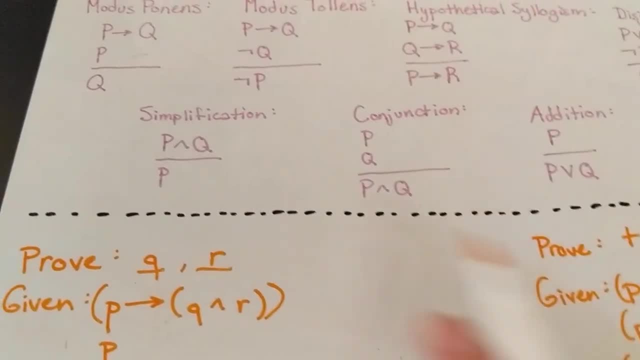 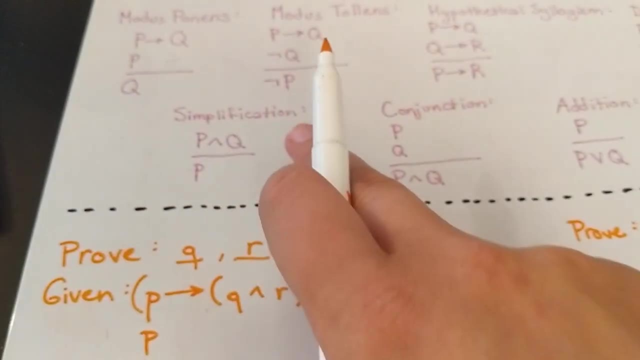 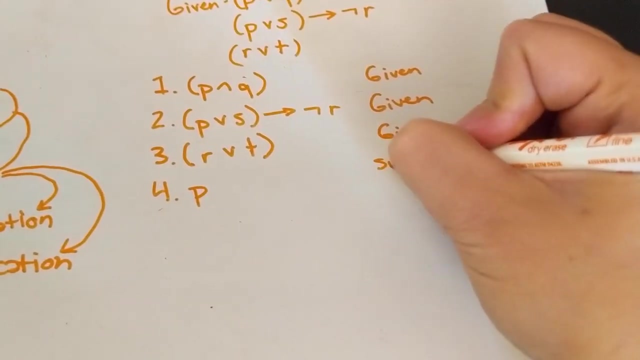 And we have a lovely rule that says: if we know that p and q is true, then we know that. or, yeah, if we know that p and q is true, then we know that p is true. So we're just going to do that and we're going to say p is true, using our simplification.